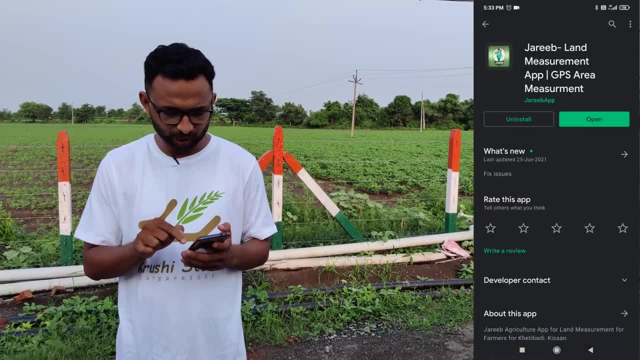 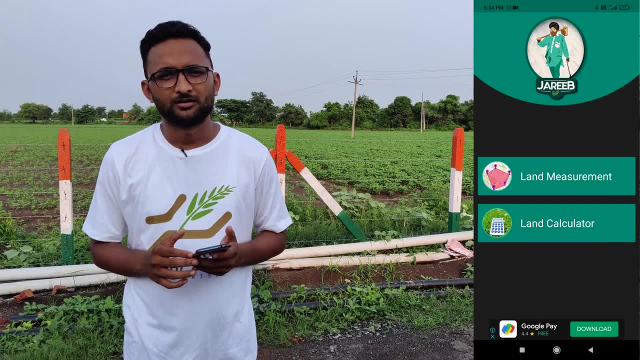 search Jareeb, and this is the first app that is shown on the Play Store. Now I have already installed this app, So I will just click on open button. After opening the Jareeb app, I see two options. The first option is land measurement and second option is land calculator. So we want to. 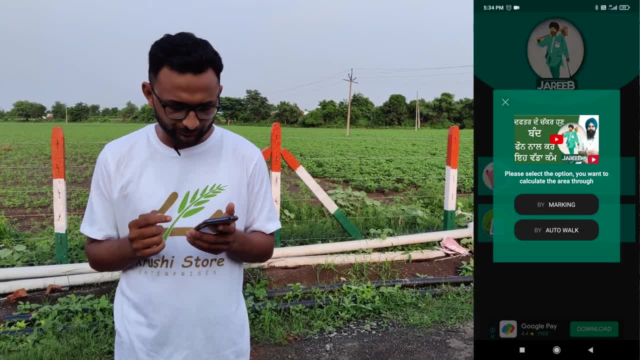 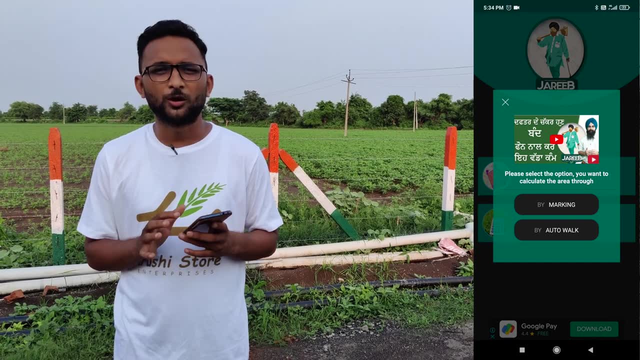 measure our land, So I will click on land measurement Now. there are two options. The first option is by marking and the second option is by auto walk. So I will choose the marking option, as the auto walk option requires me to go around the farm and then it will give me the 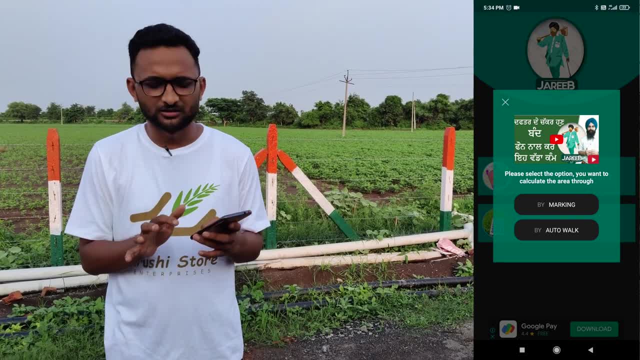 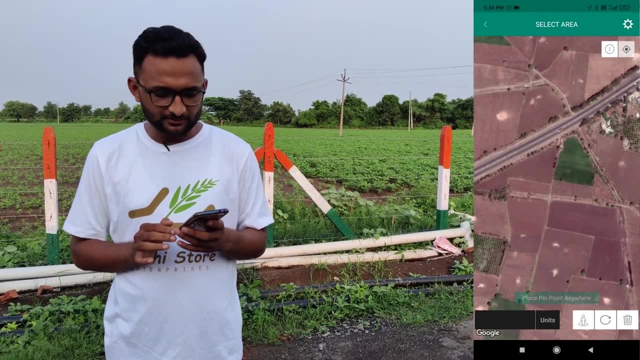 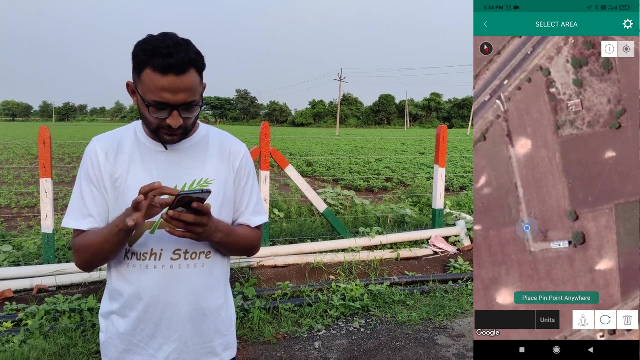 calculations, which is generally a little bit more accurate, but marking is as accurate as it can be for an estimate. So it will directly go to the place that I am standing right now and this is where I am standing and I want to calculate this portion of the land that they want to fence. So I 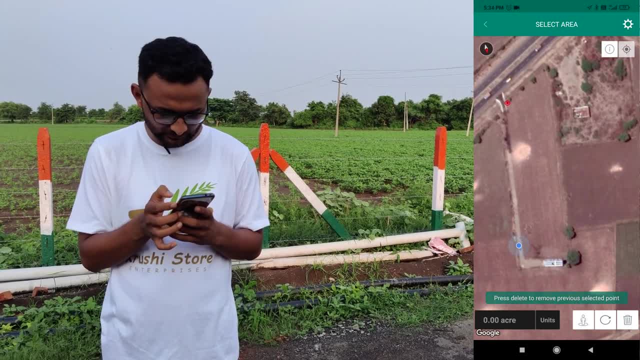 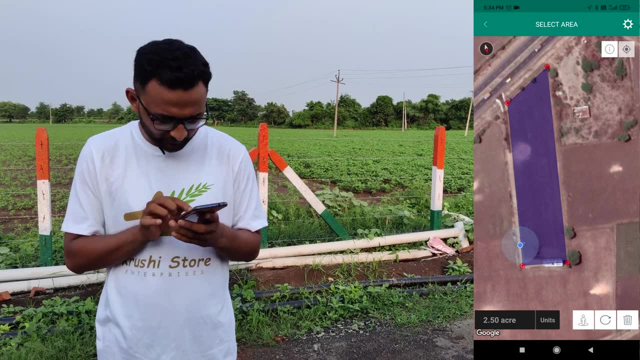 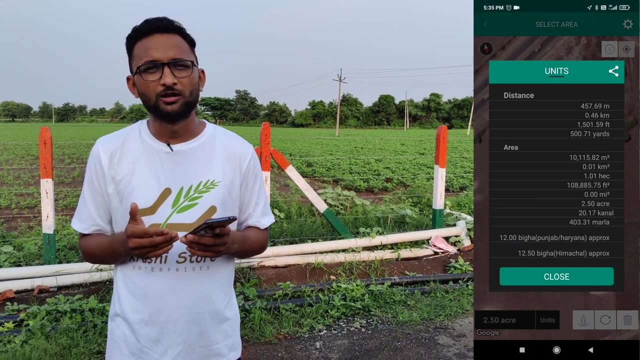 will just start adding points. So this is the first point I added. This is the second point. third, fourth, and I added four points and it has shown me that it is 2.5 acres, which is actually correct. Now, as soon as I click on the units button, it shows me all the 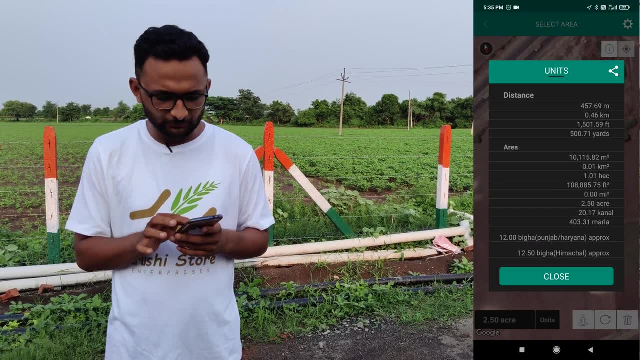 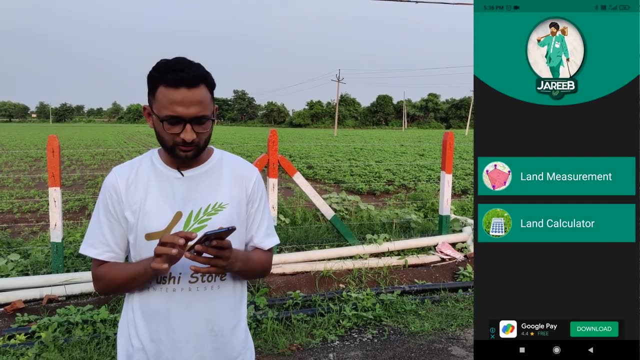 relevant information that I need to see about my farm. I also see my perimeters in meters and every other thing that I will require. Now let us go back to the main page and here I see land calculator. So if I want to convert my land from one unit to another unit, I can use this option, and this works. 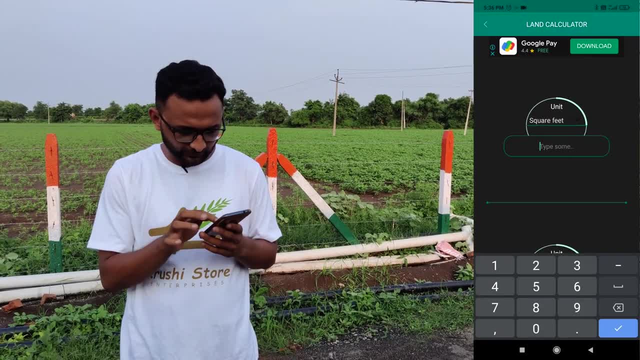 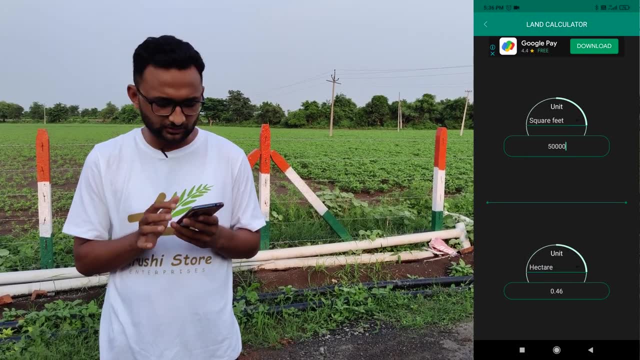 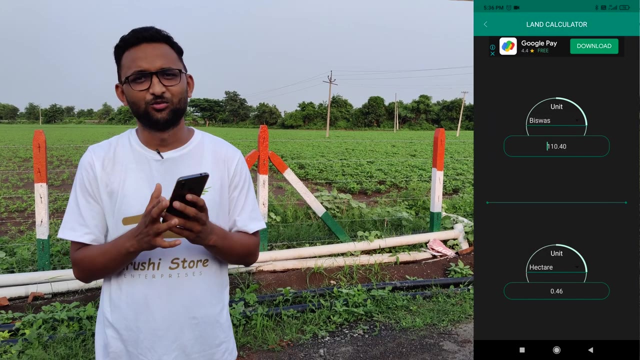 very well. So let us say that I have land of 5,000 square feet and I want to convert it to hectares. It has shown me 0.46 hectares, which is correct, and you can use this app to convert any number of units and it will work just fine every time. I think that every farmer should have this app. 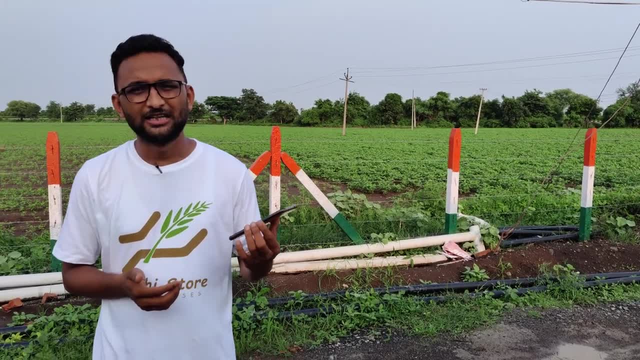 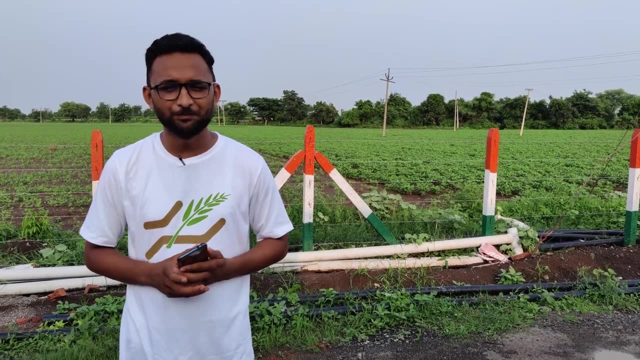 installed on their phone. It can be used anywhere, It is freely available on the Play Store and it is very lightweight, so it won't be an issue on your phone. Thanks a lot for watching. Thanks a lot for watching this Discover Agriculture video. Please subscribe to the channel for more. informative videos like this. Thanks a lot.